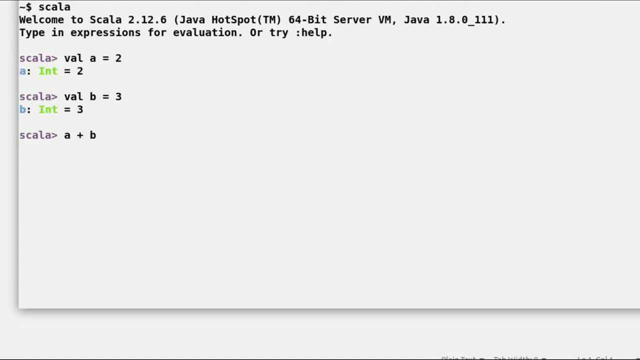 In addition, here we have a new function. This is the pure function, because no matter where you use the expression clc or deny, you will still remember a language of the building expression a plus b. in a program. you can use c instead and it won't have any side effect. 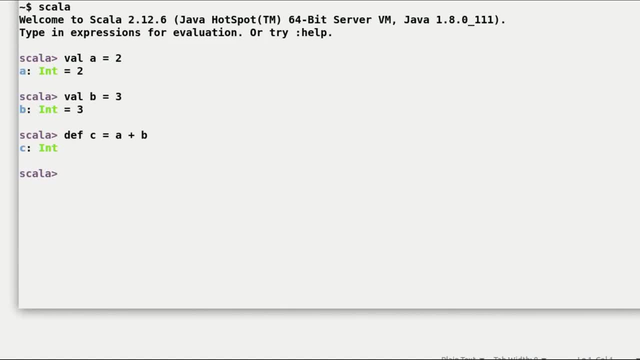 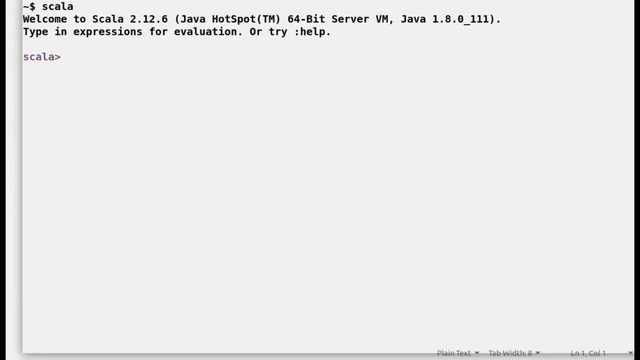 on rest of the program. The expression a plus b, therefore, is referentially transparent when you use c. This example was rather simple. Let us take a look at another example. Suppose you want to write a tool to suggest books based on Goodreads review. You may be. 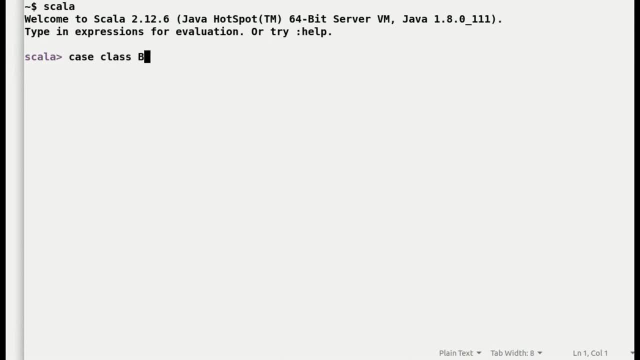 tempted to write something like this. Create a class book with name and Goodreads score First, create a method to print out the recommended book name, And the next method is to compare the books and provide the result to our first method. Let us try to execute the above code with two books, So I will pick up two of the most popular. 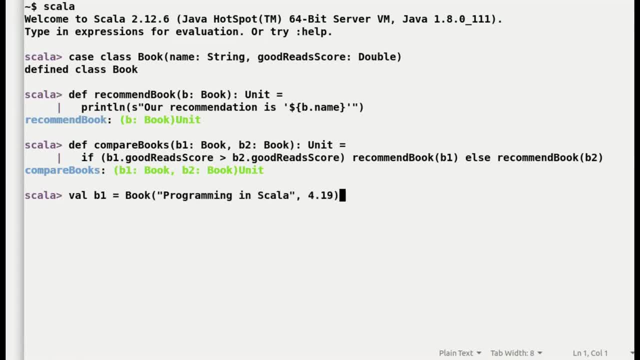 books for Scala. First is Programming in Scala with Goodreads score of 4.19 and second one is Functional Programming in Scala with score of 4.44.. And with no surprises when I pass above two books to our method, the recommended book is Functional Programming in Scala, While the above code 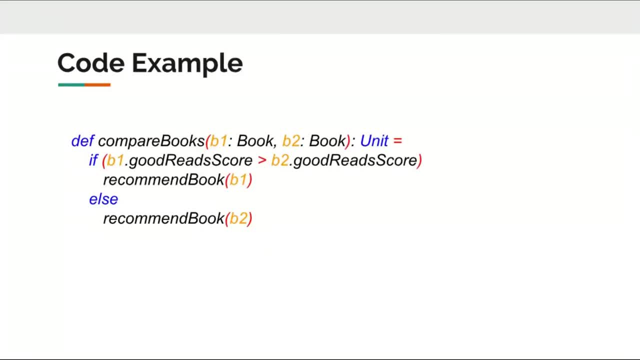 solves our initial problem. We should just do a quick test of our method and see for ourselves. We can see that the method returns Unit rather than a useful result, and it is producing a side-effect, Thus making it hard to reuse. The code can only be used to recommend. 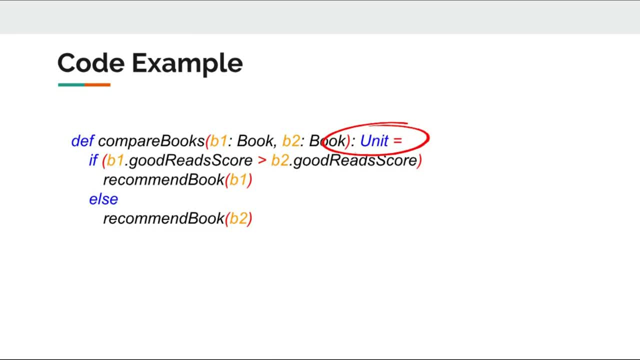 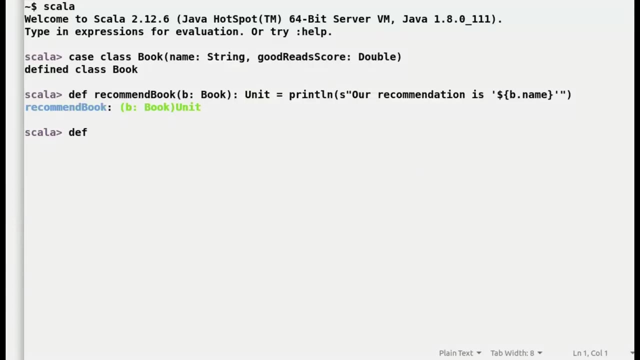 book name and nowhere else. The code can recommend a better book only between two books. What if you want a recommendation of two books? You can see that both coming from the same book out of n books. I will try and refactor the method compareBook, so instead of 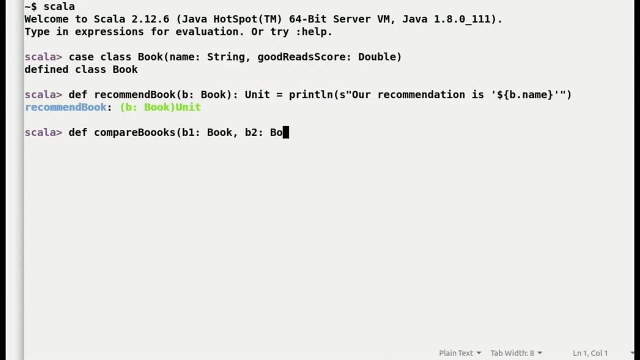 returning unit. I want to return the instance of recommended book. Let us see how this small change has made our life easier. I will create a list of popular books in Scala. The first two entries remains the same and I will enter another entry of Scala for impatient. Now I will show you something really useful. 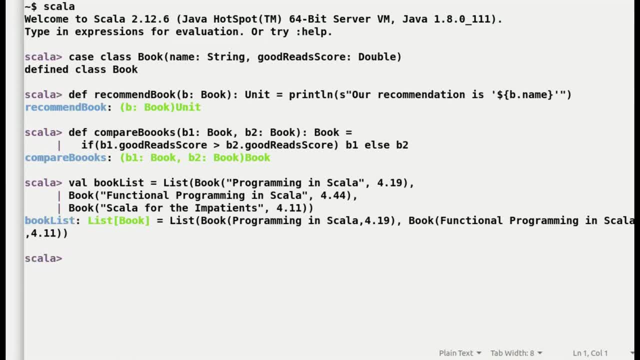 and really fun. I want to show you the use of reduce left. Reduce left will compare all the elements of the list to fetch the final result. Here it will compare all the books in the list to get a book with best reviews. If you don't know about reduce function, don't be bothered about it, Try to. 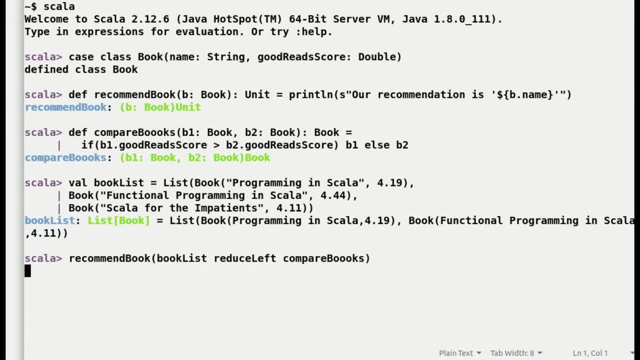 understand the concept of pure functions. here I have created another detailed video to explain reduce and here, when we execute the code with no surprises, the recommendation is functional programming in Scala. Though all the books in the list are great resources and you can pick up any of them to explore Scala in great 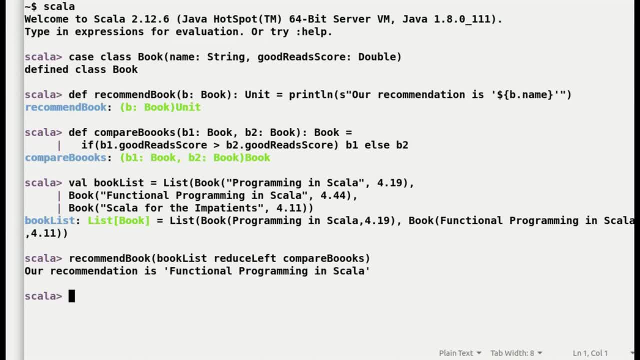 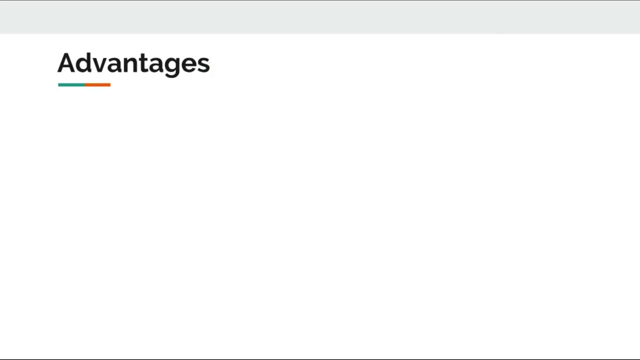 detail. So here we got rid of any side effects and we got a result with expected behavior. I hope you enjoyed this concept of pure functions. The concept is really useful. So altogether, a pure function has many advantages. These properties give us an unprecedented ability to reason about our code, For example. 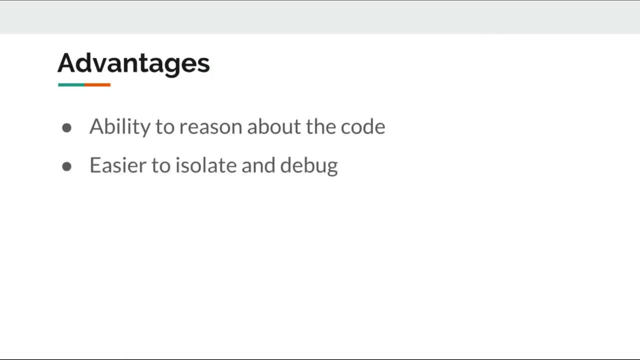 any input, validation or calculation is easier to isolate Caching. the result is possible when functions are deterministic and interactions with the world becomes easier to control and test. Let us drill down on pure functions once again. Pure functions are independent of any other changes in the program. They